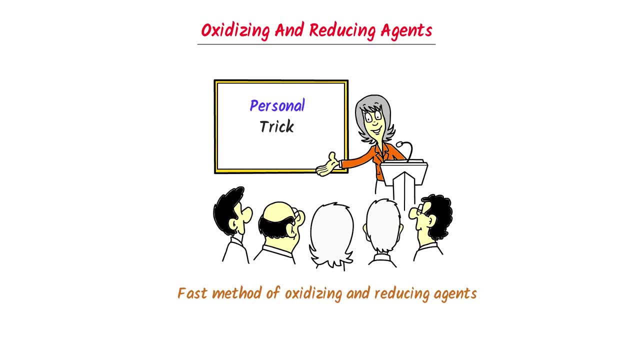 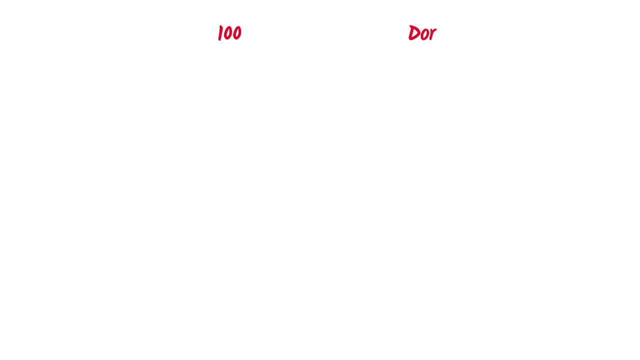 learn oxidation and reduction. In the previous video we have already learned that oxidation is 100 and reduction is door. Here 100 stands for increased oxidation- number is oxidation and door stands for decreased oxidation- number is reduction. For example, consider sodium atom. 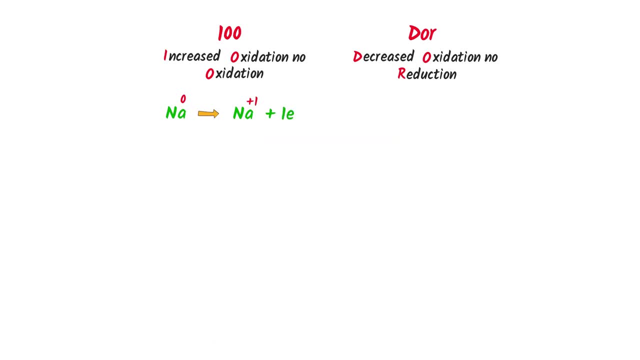 Now this sodium loses one electron to become positive ion. Here we can see that the oxidation number of sodium increased from 0 to positive 1. So we say that sodium is oxidized. Now listen carefully. This lost electron is gained by the chlorine atom to become 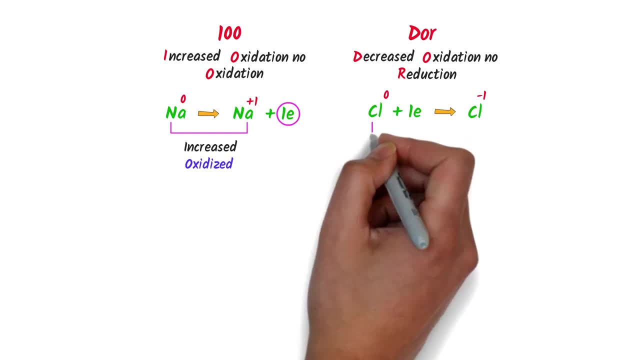 negative ion. We can see that the oxidation state of chlorine decreased from 0 to negative 1.. So it is reduced. Now let me ask you how sodium is oxidized and chlorine is reduced. Well, the answer is simple: It is due to the availability of two opposite. 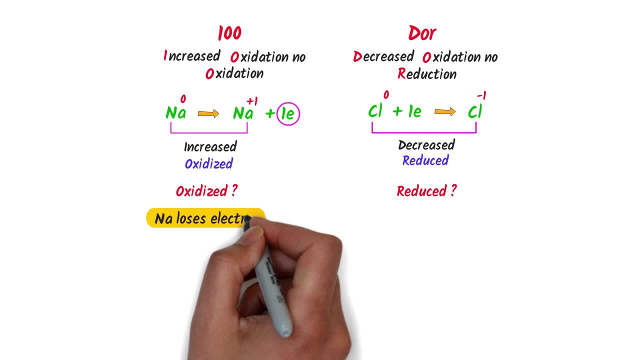 species- I mean sodium- loves to lose electrons and chlorine loves to gain electrons. Let me repeat this important point: Sodium loves to lose electrons and chlorine loves to gain electrons. So it is due to the opposite nature that sodium loses electron and get oxidized. 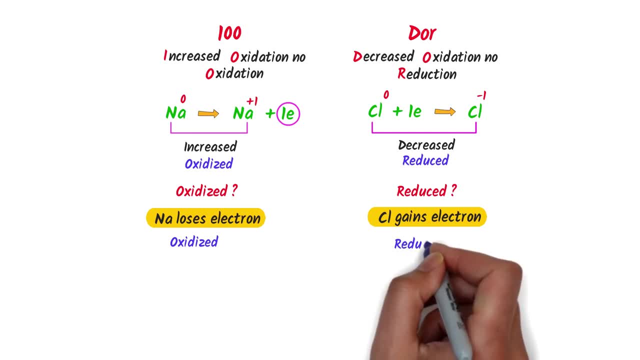 while chlorine gains electron and get reduced. Now listen carefully. Sodium is oxidized by chlorine because chlorine forces sodium to lose electron, So we call sodium as reducing agent. Secondly, chlorine is reduced by the sodium because sodium forces chlorine to accept electron, So we call chlorine as oxidizing agent. 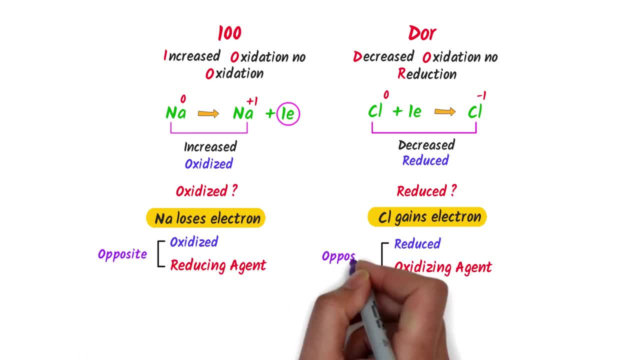 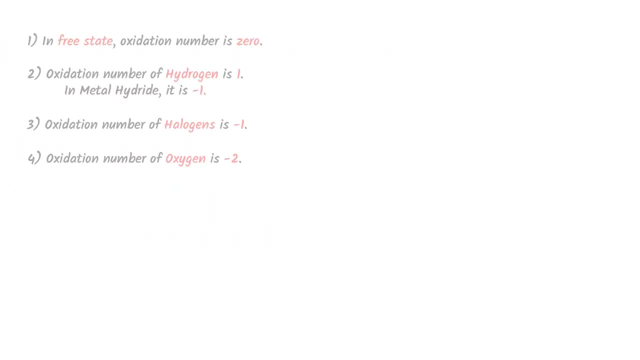 Here the easy trick is to use opposite words: Sodium is oxidized by chlorine, because chlorine is oxidized, so it is reducing agent, while chlorine is reduced, so it is oxidizing agent. Now let me teach you some real life examples. I will use these four rules to instantly spot. 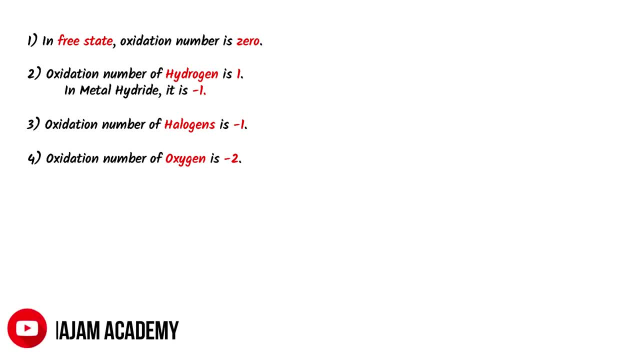 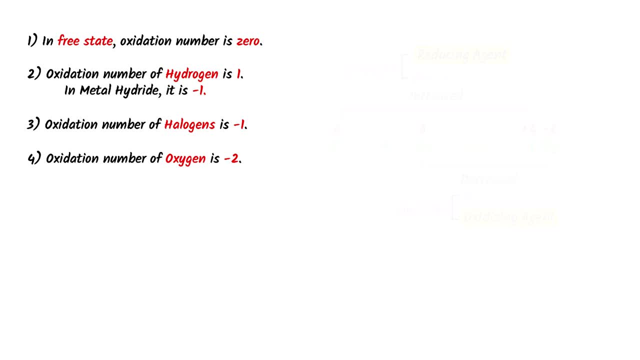 oxidizing agent. Secondly, consider hydrogen gas plus oxygen gas react together to form water. We know that hydrogen gas and oxygen gas is in free state, so I write zero oxidation state for hydrogen and zero oxidation state for oxygen. In case of water, there are two atoms of hydrogen and there is one. 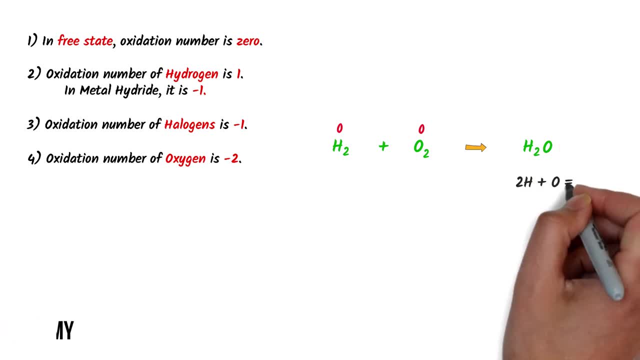 atom of oxygen. So I write: 2H plus oxygen is equal to zero, because the overall charge on water is zero. We know that the oxidation state of oxygen and its compound is negative two, So I write: 2H plus negative two is equal to zero, or. 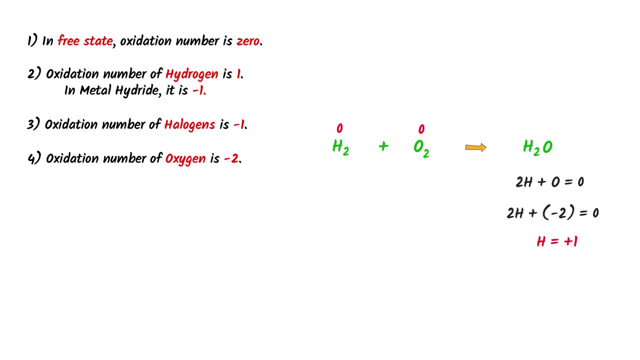 H is equal to positive one, So the oxidation state of hydrogen is positive one and that of oxygen is negative two. Now we can see that the oxidation state of hydrogen increased from zero to positive one, so it is oxidized. The trick is to use opposite world. I write. 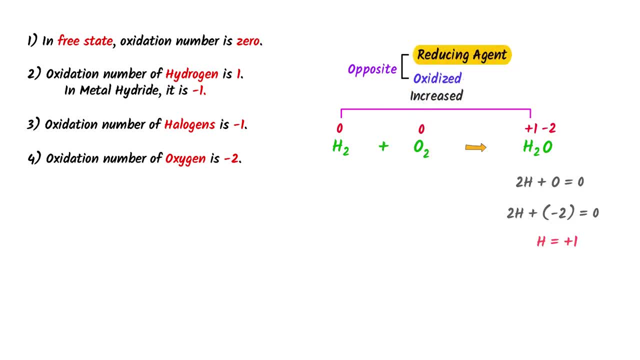 reducing agent. Secondly, we can see that the oxidation state of oxygen decreased from zero to negative two, so it is reduced. The trick is to use opposite world. I write oxidizing agent. Thus here, hydrogen gas is reducing agent and oxygen gas is oxidizing agent. 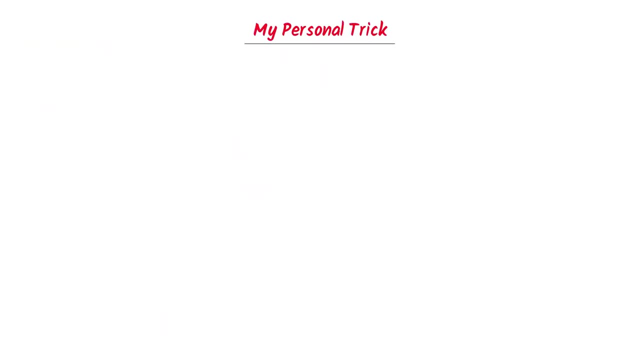 Finally, let me teach you my personal and easy trick to remember the list of common oxidizing agents and common reducing agents. In case of common oxidizing agents, I write HMCC, no halogen, 2H2K for computer science. Here these all are oxides like hydrogen peroxide, manganese oxide, calcium oxide, chromium oxide. 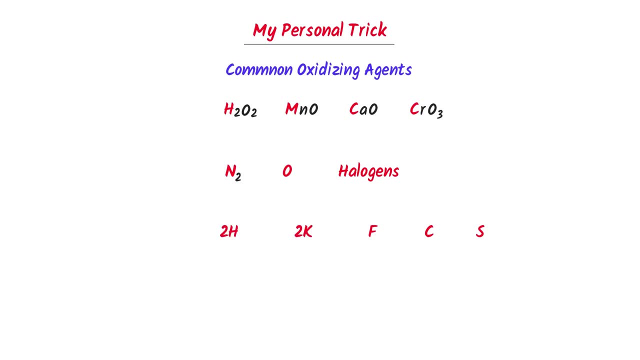 Now, here N stands for nitrogen gas, O stands for oxygen gas, while halogens like fluorine gas, chlorine gas, bromine gas and iodine. Here one H stands for sulfuric acid and another H stands for nitric acid, HNO3,, while in case 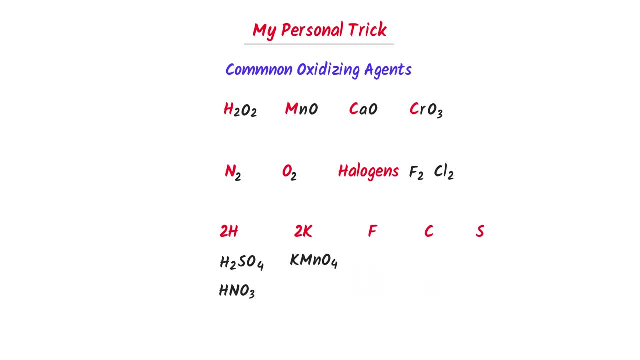 of 2K. one K stands for KMnO4,, while the other K stands for potassium dichromate. Here F stands for iron chloride, this C stands for carbon dioxide and this S stands for sulfur trioxide. Thus, using my personal trick, you can easily learn the list of common oxidizing agents.